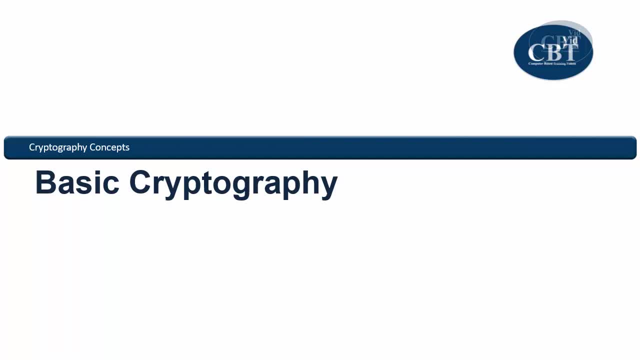 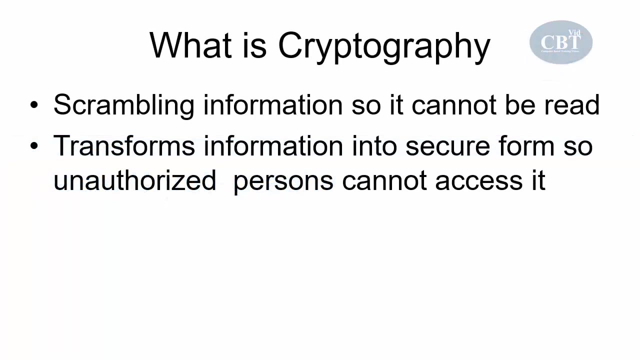 Now, that message could be something that a general is sending to another general, or it could be something that you know a person is sending to another family member. So cryptography is an answer to that concern. Now, what is cryptography? It's basically the art of transforming a message into a secure form. so 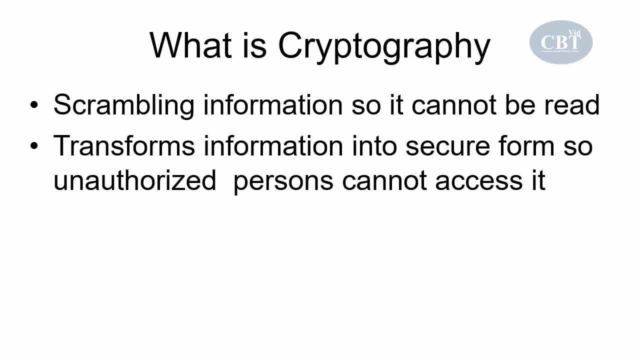 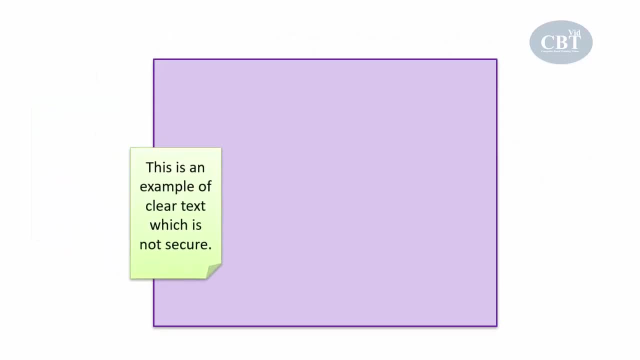 that someone unauthorized cannot read the content of the message. So we're transforming a clear text message to some gibberish that is not readable and understandable by people. So you have a plain text, a readable message, and you send that readable message through some processes. 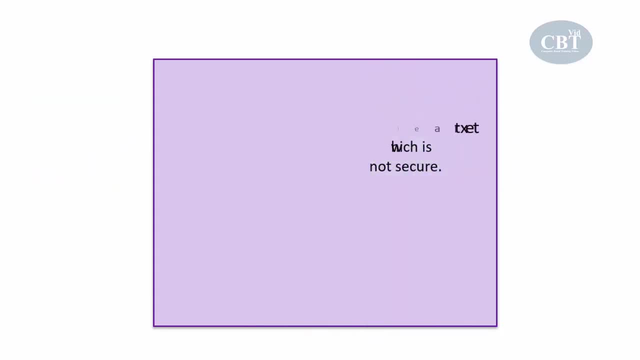 and in that processes the message gets converted to something which is not readable. to some gibberish that if somebody gets access to that message they cannot read it. So that message which is not readable is called ciphertext. So I have plain text. I send it through some processes. 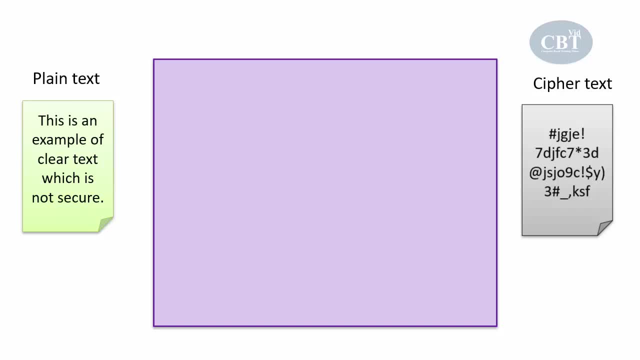 and then I get ciphertext. Now, during this process, you're basically encoding your message or you're enciphering the message. Now, when the recipient receives this message, they cannot read the message either. So what they do is they have to send that message through the same processes and get the message. 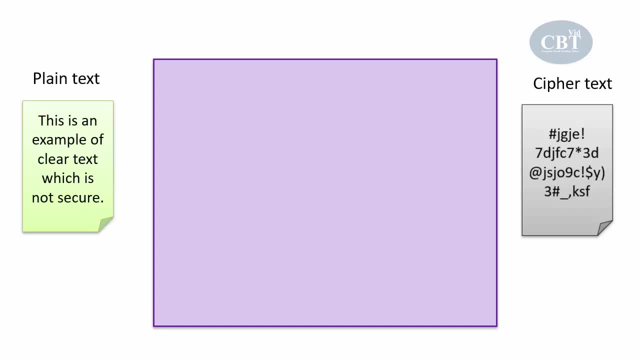 converted back to something which is readable, which we call it plain text. Now this process of converting message from plain text to ciphertext is called encryption algorithm. So the whole process is called algorithm And when you use it for encryption, encryption algorithm. Now the problem with this process of converting plaintext to ciphertext: 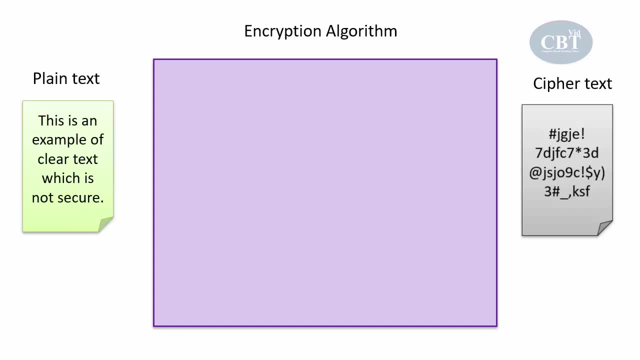 using an encryption algorithm is that if an unauthorized person gets access to the ciphertext and if they come to know what algorithm you have used, then nothing stops them from sending your ciphertext through the same algorithm to get the plaintext and read the content of the message. 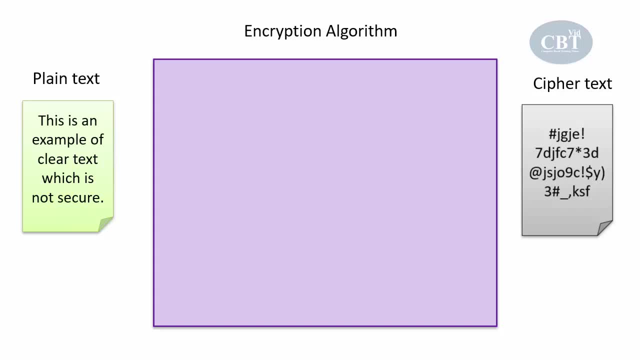 Now to address this issue. they have come up with a key. So when you're sending your message- the plaintext- through the encryption algorithm, you send that key to that algorithm too. So you use the key and plaintext together in that algorithm to convert the plaintext message to. 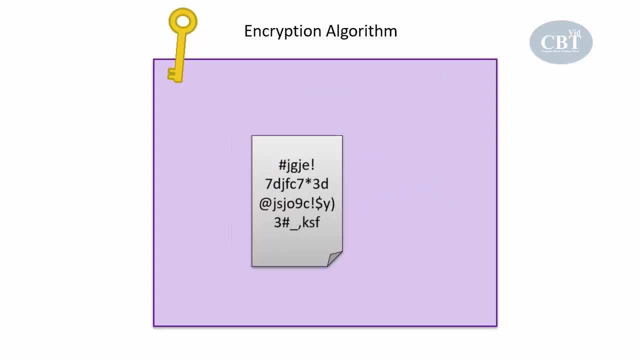 some gibberish or to ciphertext. So I'm not going to say gibberish anymore, I'm going to say ciphertext text from now on. so now i have the cipher text and i use a plain text with the algorithm and the key. 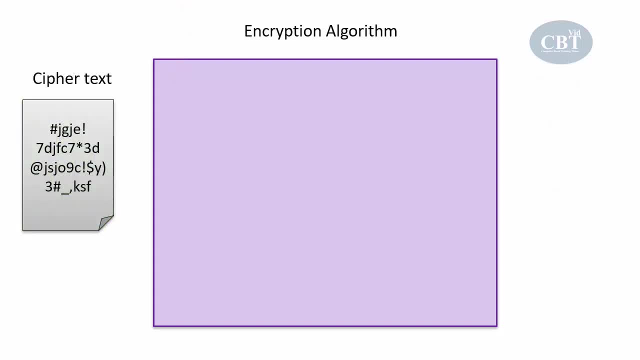 to get that cipher text. so, as i mentioned before, if you want to convert the cipher text to plain text, then you have to send that cipher text and the key to the same algorithm and get your text converted back to plain text. now the algorithm, when it's used for encryption, we call it encryption. 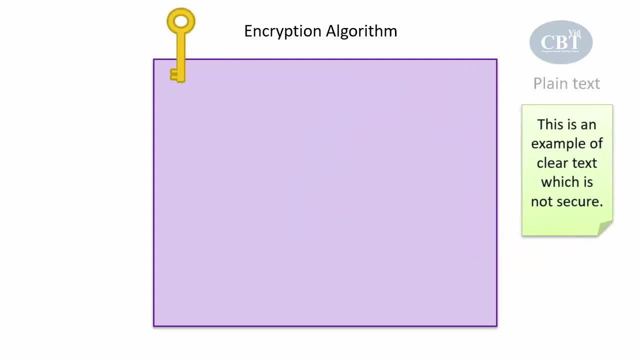 algorithm, and when we use the same algorithm for decryption, we call it decryption algorithm. all right, now that you know that we have an algorithm that can be used for transforming uh plain text to ciphertext or ciphertext to plain text, you need to know that we have different types. 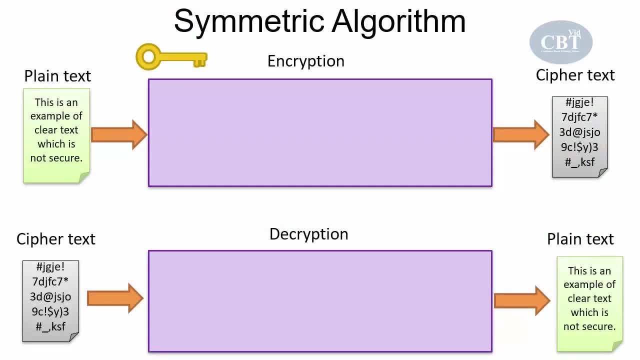 of encryption algorithms. we basically have two types of encryption algorithms. we have two types of encryption algorithms. one is symmetric algorithm. in symmetric algorithm, you use one key to transform the plain text to cipher text and you use exactly the same key to transform the cipher text to plain text. the second type of algorithm is asymmetric algorithm. 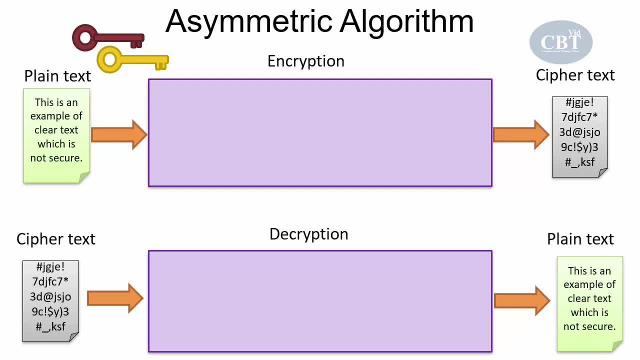 now in asymmetric algorithm you have two keys. you use one key for encryption and you use gehört formatting and brace沙네, Collette, alchol, property application, time management, other key for decryption. if you use first key for encryption, you have to use the second key. 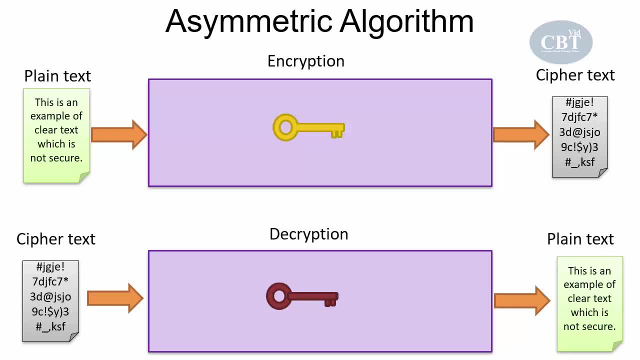 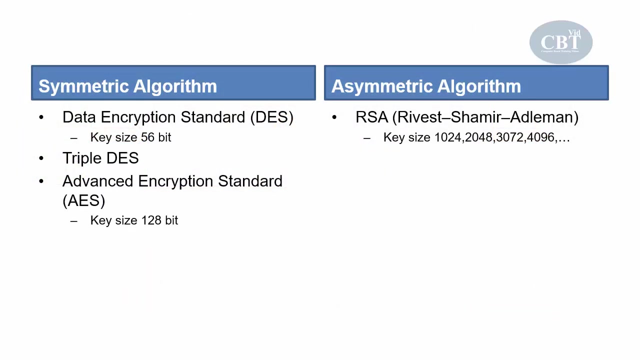 for decryption. you cannot use the first key for decryption and if you use the second key for encryption, then you have to use the first key for decryption. that is the difference between these two algorithms. now we have so many different algorithms that are categorized under symmetric and asymmetric. so if you look at this slide, we have data encryption standard. that's an encryption. 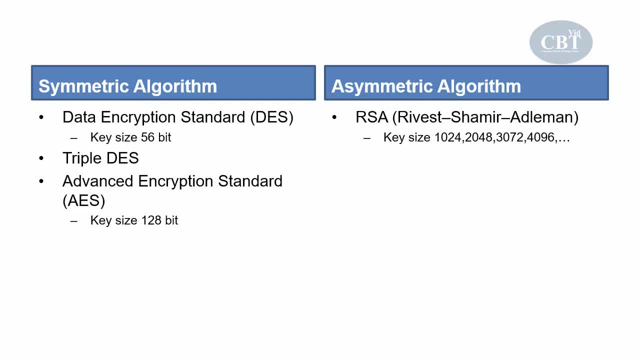 algorithm, which is a symmetric algorithm. we have a triple des, which is basically data encryption standard, but you use it three times and the reason that you do that is to make the algorithm more stronger, more secure. another type of algorithm that we have which has been widely used nowadays: 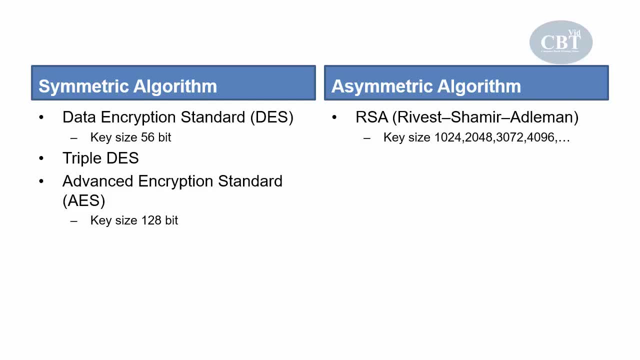 and it's the most secure one is called advanced encryption standard or aes. if you look at all these algorithms, you can see that they have different sizes of keys that can be used with. for example, data encryption as a standard has a key of 50- 56 bit, so that means when you want to use this. 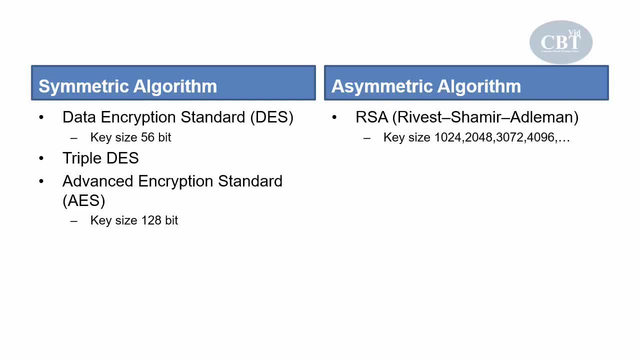 algorithm, the key that you're going to use is going to be 56 bits of key. you send that key and your text to this algorithm to get the ciphertext. when it comes to advanced encryption standard, it can work with multiple sizes of keys. you can have a key of size, 128 bit or 256 bit, so the larger the 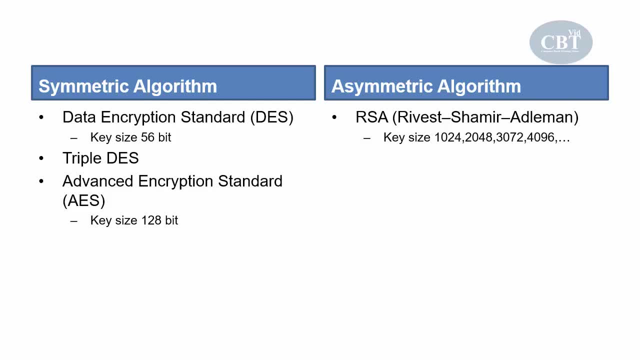 size of your key, the stronger your encryption can be. and the difference between this symmetric algorithm is basically the mathematic procedures that they use to convert the plaintext to the ciphertext. now, if the algorithm works in this way, if the algorithm has a literal size of 218 bit plus 1 meter, 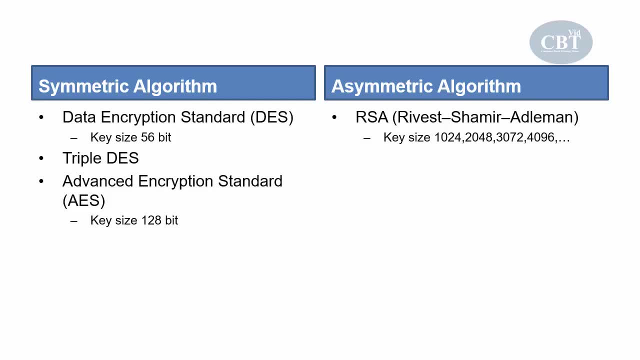 plus one second, four, hebrew, that programming ec, which you actually see in notebook we have created here by these two ciphertexts, the. the requires two ciphertext. now if the mathematic procedure is very sophisticated, then that makes the algorithm more powerful, stronger algorithm, and if the key size is longer, that makes even the algorithm strong. now on the right side of the screen you can see we have an asymmetric algorithm. 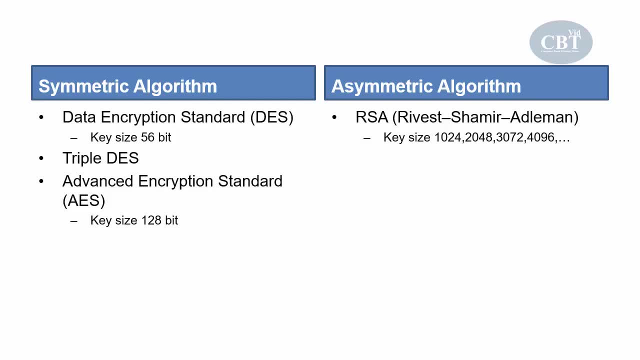 is being misused. Bernie urg are for quite a long time. So, as you can see, the size of the key with asymmetric algorithm is significantly bigger than what we have in symmetric algorithm. Now you may be asking that, since asymmetric has larger key size compared to symmetric algorithm, why do we need to use? 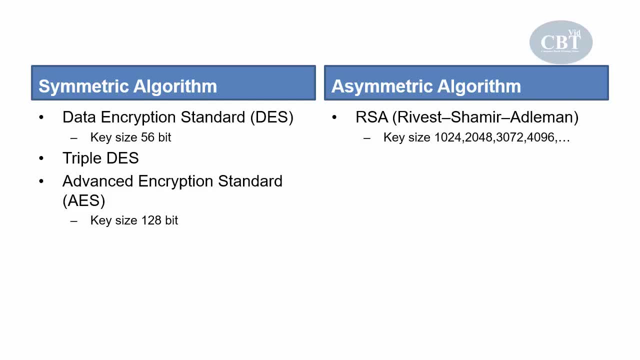 symmetric algorithm. Why don't we use asymmetric algorithm for everything? Well, one reason for that is the resources that you need to handle asymmetric keys, For example. if you're using asymmetric key, the speed of the communication might be much slower than symmetric algorithm. 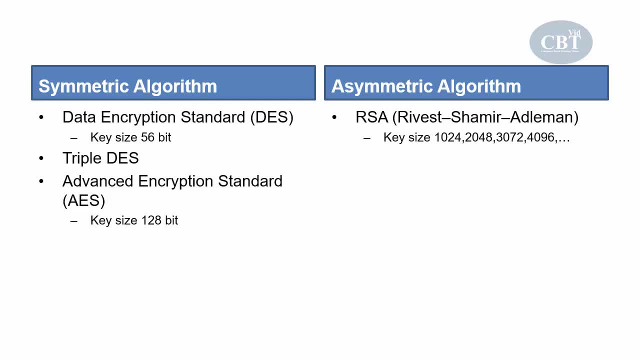 and you need a lot of CPU power to handle asymmetric algorithm. Imagine you're accessing a website using a secure HTTP protocol and if that website uses asymmetric algorithm all the way, then the communication with that website is going to be really slow and you will see that your CPU usage 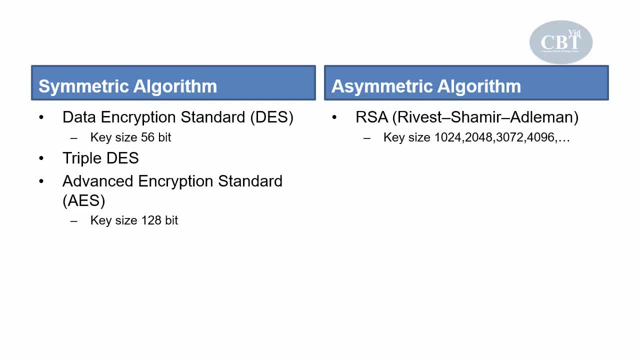 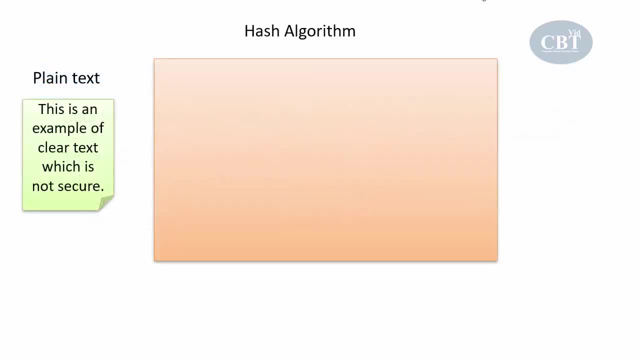 is going to be really high to handle all these encrypted traffics using asymmetric algorithm. The third type of cryptographic algorithm that we have is called hashing algorithm. Now, the difference between hashing algorithm and the previous two is that hashing algorithm is a one-way algorithm, So when you encrypt your message, you cannot decrypt it back. 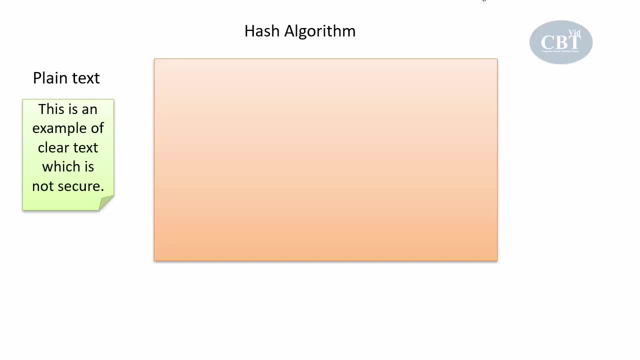 And technically, with hashing algorithm you're not really encrypting your message. The result of hashing algorithm is called a digest or a digital fingerprint or a hash file. So when you send your message through a hashing algorithm, it goes through some calculations, some mathematical. 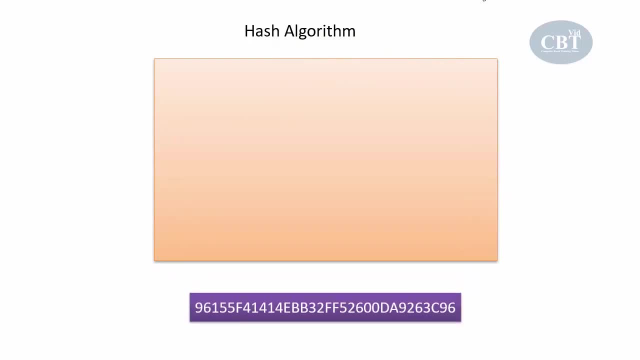 procedures and the end result is going to be a digest of the file or a hash of that file. Now you may be asking: why do we need such an algorithm If you're using asymmetric algorithm? if I cannot decrypt the message that I encrypted, then what's the point of using this algorithm? 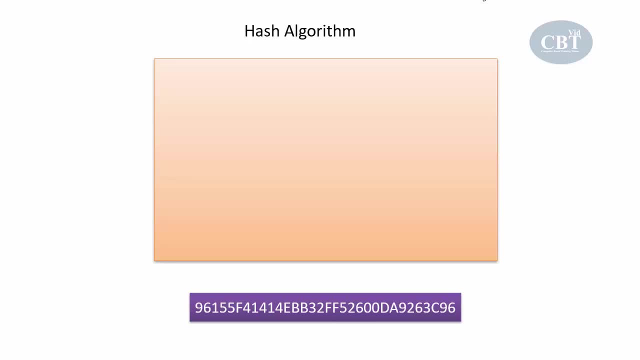 Well, that's a very good question that I ask for you. In the symmetric and asymmetric algorithm, you are encrypting a message, So these algorithms protect the confidentiality and integrity of the message. Hashing algorithm is just for the integrity of the message, Because in hashing algorithm you don't need to have a key. 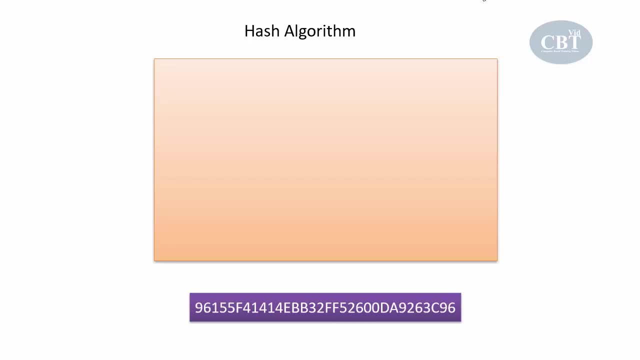 You just need to know the algorithm. So when I send a message to someone, I just tell them what hashing algorithm I used, And then they can use the same algorithm to check the integrity of the message that I sent to them. Now the way that this works is that: 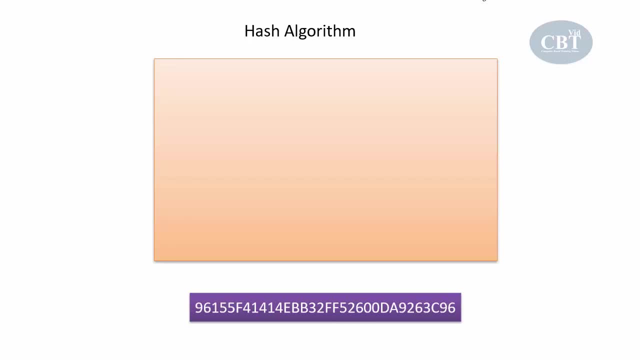 when I want to send the message to someone else, I calculate a hash of that message And then I send the message with the hash file to the recipient. Then, when the recipient receives that message, they're going to use the same hashing algorithm to. 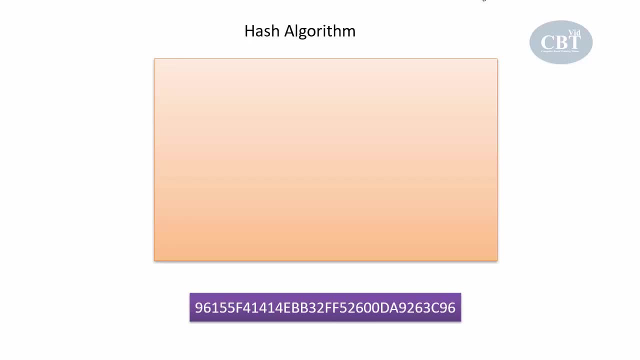 generate a hash of that file. If the produced hash is exactly the same as the one that I sent to them, then they know that the message is intact and nothing with the content of that message has been changed. So when you use this algorithm, you don't really care that someone sees the content. 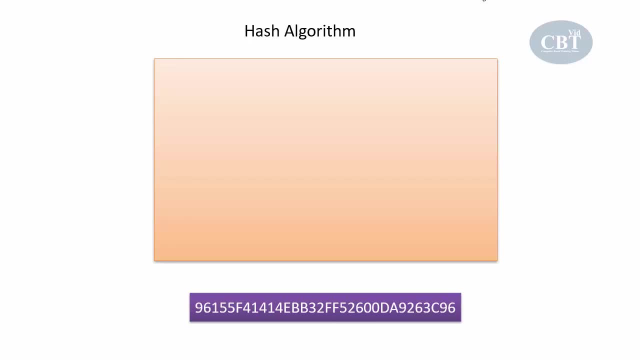 of your message. What you care is the recipient receives the exact message that you sent to them. Now, one thing about the hashing algorithm is that whether you send a letter, a page or 10 volume book as an input to the hashing algorithm, the end result is going to: 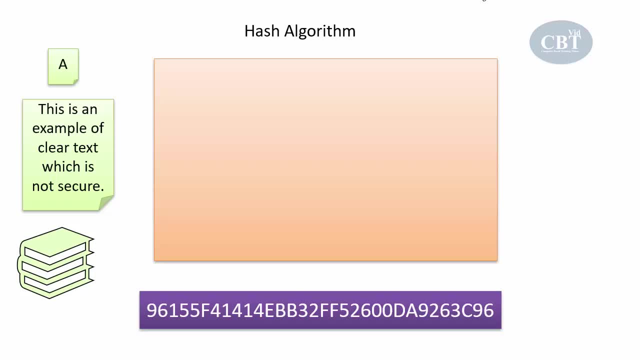 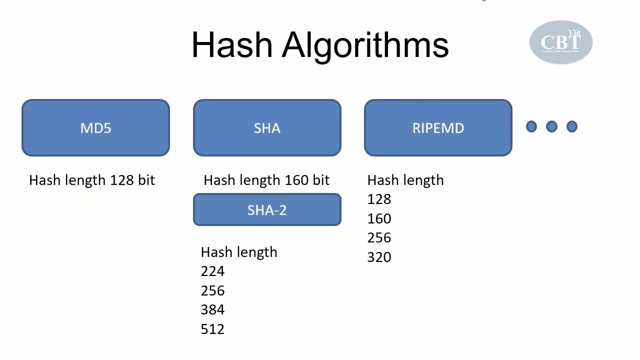 be the same size. Now, the same way that we had multiple algorithms with symmetric and asymmetric algorithms, in hashing also we have different types of algorithms, And the main difference between these different algorithms is in the mathematical calculation of the digital fingerprint or the hash file, One of the earliest and 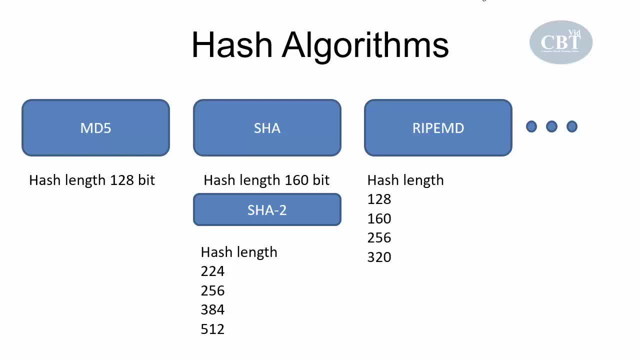 most popular hashing algorithm is MD5, or Message Digest 5.. Now the 5 is the version of this algorithm. So it started from Message Digest 1 and 2, and then it reached the Message Digest 5.. As you can see, 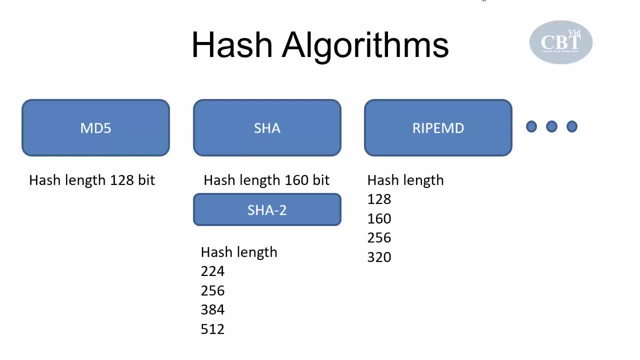 the length of the hash file that is generated by Message Digest 5 or MD5, is 128-bit. So, as I said, whether you send a letter or a page to this hashing algorithm, the end result is going to be 128-bit. 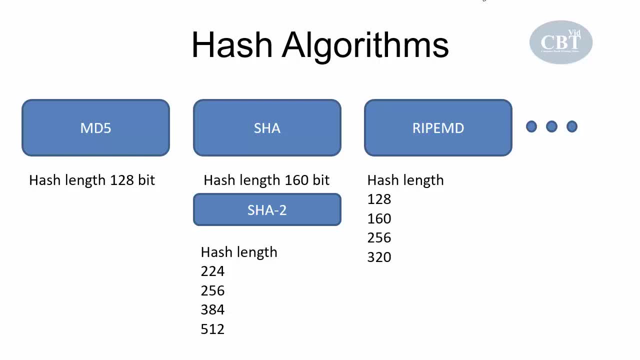 Now, later, some vulnerabilities were found with MD5, and then SHA-1 was introduced as a more secure hashing algorithm. As you can see, SHA generates a 106-bit hash file, So whatever you send to SHA-1, the end result is going to be 160-bit. And then. 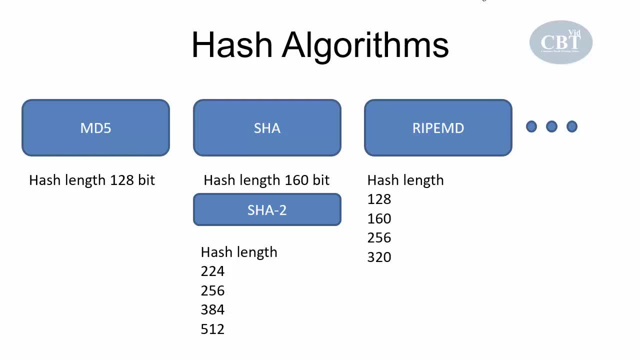 SHA-1 also was found to be a little bit vulnerable, and then SHA-2 was introduced as a more secure version of SHA-1.. And SHA-2 generates different hash sizes. As you can see, the hash length can be 224-bit all the way to 512-bit. 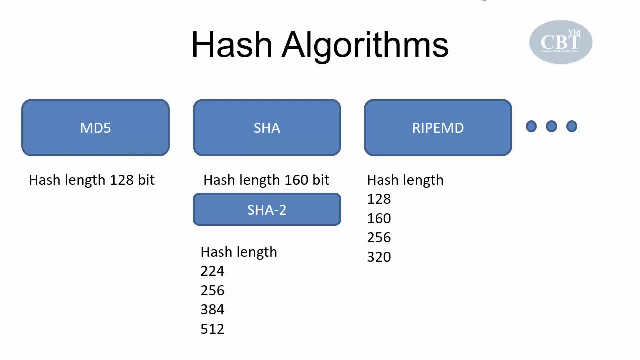 Recently, SHA-3 has been introduced as the most secure version of SHA-2.. Another type of hashing algorithm that we have is called Race Integrity Primitives Evaluation Message Digest, or RIPEMD. Now, this algorithm was created by RACE, which is a European Union. 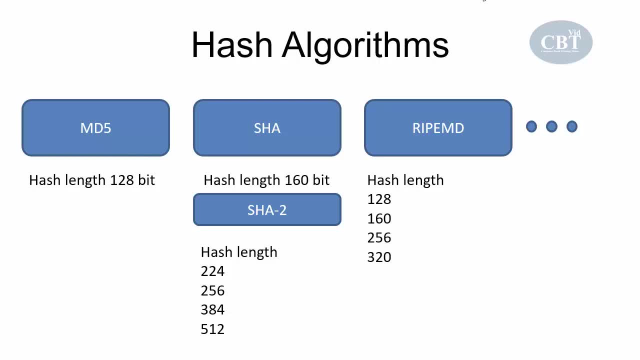 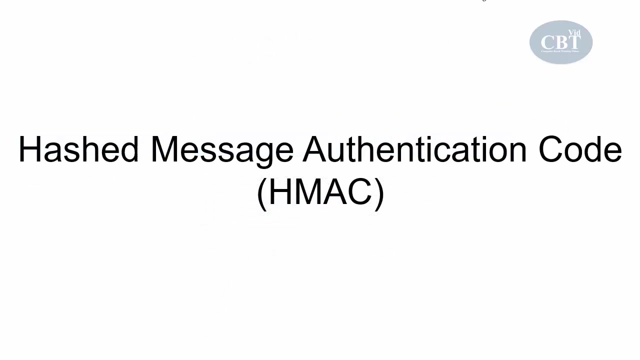 affiliated organization. As you can see, this algorithm also generates hash files in different sizes. Now there are other hashing algorithms out there, But what you see in these slides are the most common and popular ones. One of the usage or applications of the hashing algorithm is in hashed message authentication. 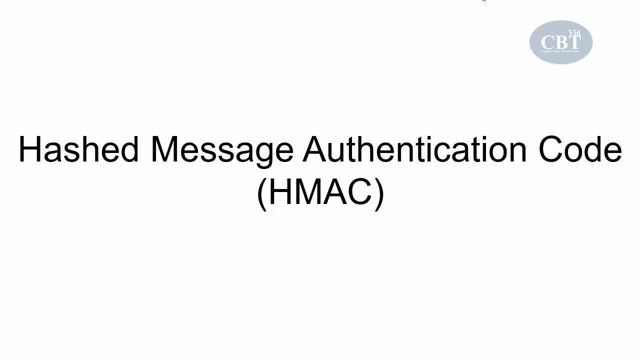 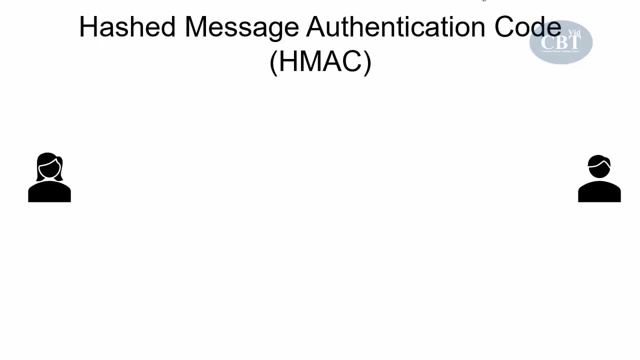 code. As the name says here, this hashed message authentication code is used for authenticating a user. Let me explain it works. let's say we have two users, alice and bob, and these two, uh, when they send the message to each other, they want to make sure that the message came from the right person, so they want. 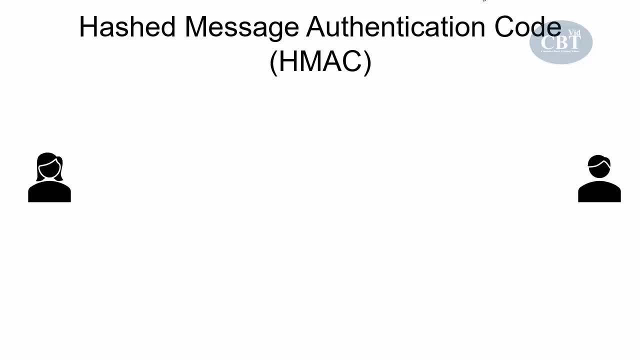 to use hmac for authenticating each other. now both of these users have same secret key, so they both agreed on the same encryption algorithm and they generated as the same secret key to use with that symmetric algorithm when they exchange messages. now, let's say, alice want to send a message to bob. 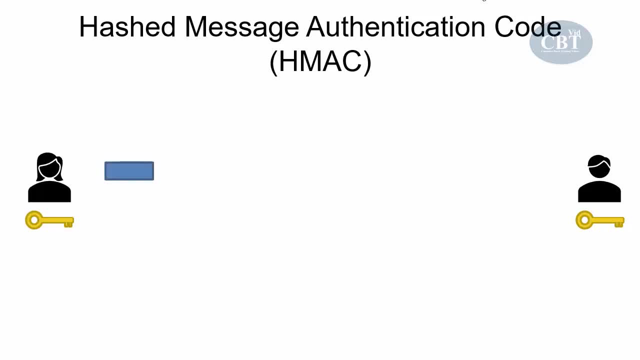 so she uses the same secret key that they have to encrypt that message, and then she uses a hashing algorithm to generate a hash file for that encrypted message and the key, the secret key that she has. the end result is going to be a hash file. now, next thing that she's going to do is send this. 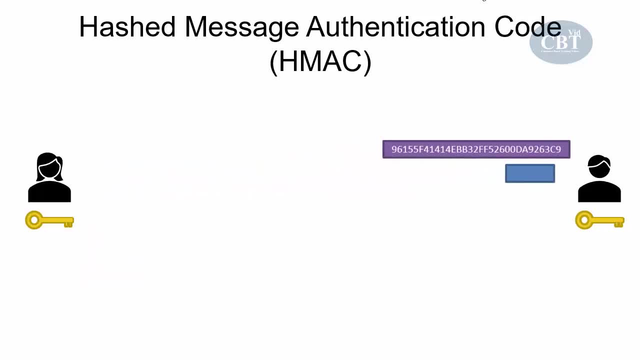 hash file, and then she's going to use the same secret key to encrypt that message. and then she's going to send the same encrypted message to bob when bob receives the message. before decrypting the message, he's going to make sure that the message actually came from alice. so the way that 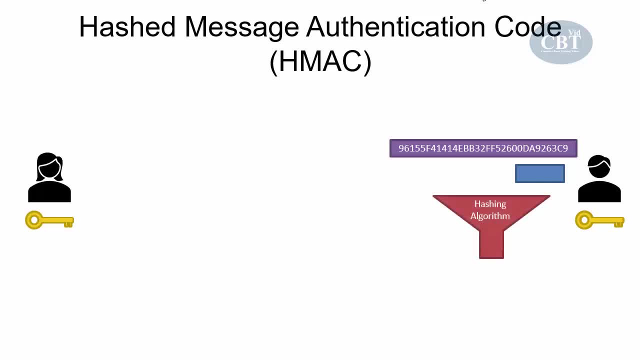 he's going to do that is by using the same hashing algorithm. he's going to send the same encrypted file and the secret key that he has to that hashing algorithm to generate a hash file. then when he generates that hash file, he's going to compare that hash file with the one.